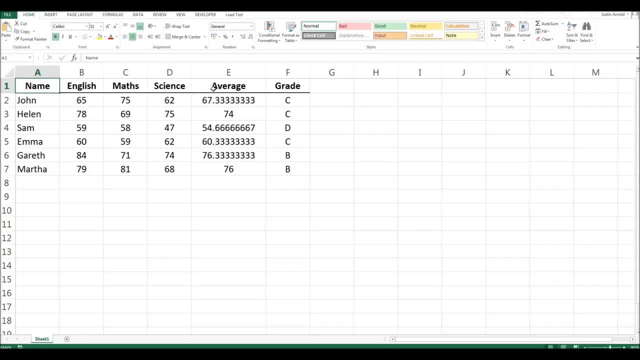 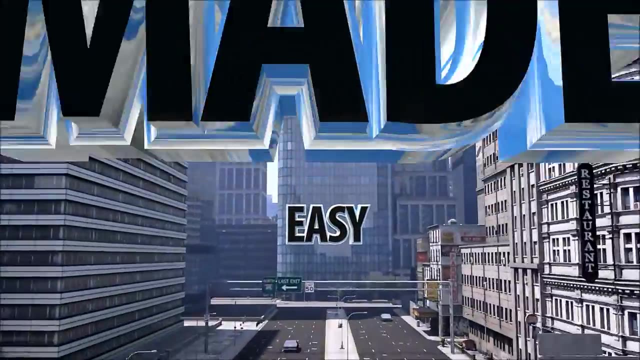 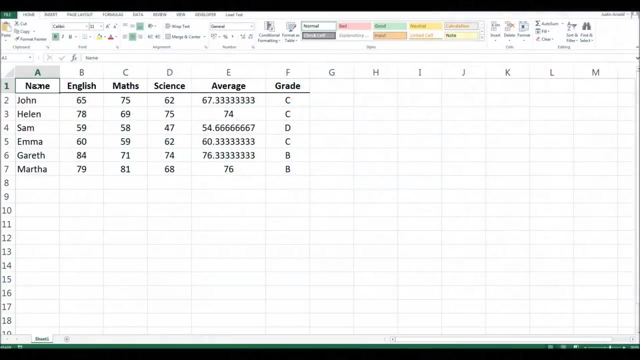 Hello. so you have a spreadsheet with a column like this, containing more decimal places than you know what to do with. How can you round those numbers to a set number of decimal places? If in your spreadsheet you end up with formulas that generate numbers that have huge number of decimal places and it gets unwieldy, it gets scruffy, untidy, how can you round those numbers so that they are a set number of decimal places? 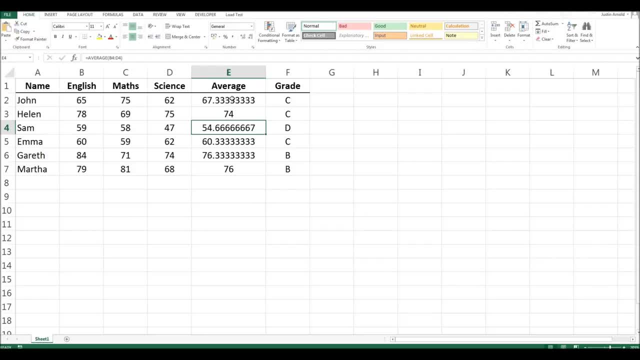 So one or two decimal places. It's actually quite simple and to demonstrate this I'm going to insert a new column and put a function in this column which takes these numbers and rounds them to two decimal places. The function itself is the round function. 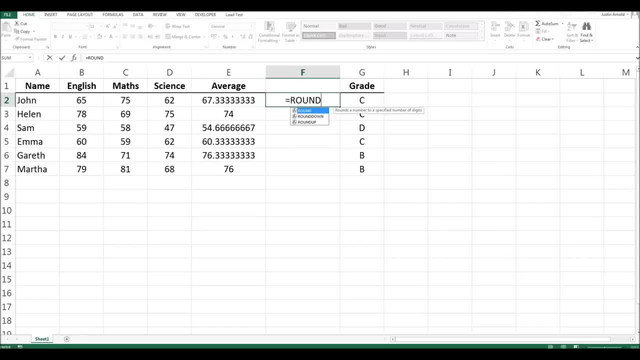 So we simply type equals and then round, open up our brackets and select the cell we want to round. that's E2. And then we're going to round. And then we're going to round. We have to just put a comma and the number of decimal places we want to round that number to. 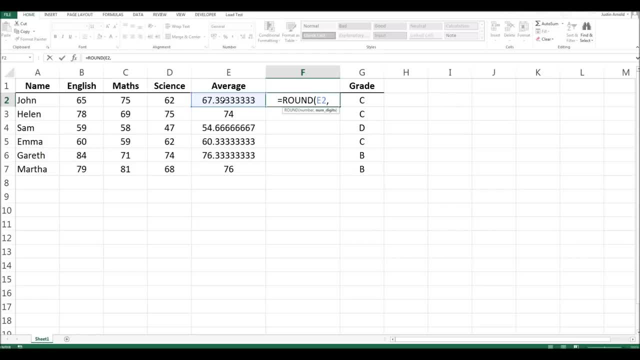 So let's say we want this number to be rounded to two decimal places. we type a, 2 and then of course close our brackets. So equals round this number to two decimal places. If we press enter then we can see we've now rounded this number to 67.33. 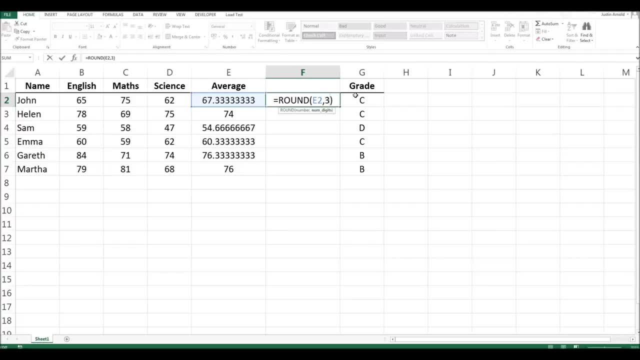 If I quickly change that 2 to a 3. We can see we're rounding that number now to three decimal places. We could do the same for 1.. I'm going to keep that to 2 for the moment and replicate this formula down by grabbing the box at the bottom right corner. drag that down so that all of these numbers are now rounded to two decimal places. 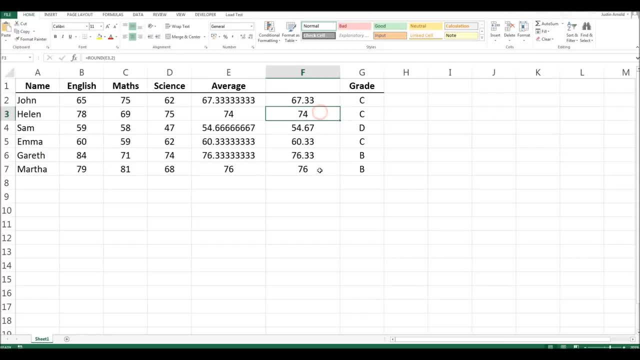 Except of course they're not, Because these two numbers were not. they did not have decimal places at all, They were whole numbers. Now this can look a little scruffy. Some people prefer it if all the numbers have the same number of decimal places, regardless of whether they need decimal places or not.